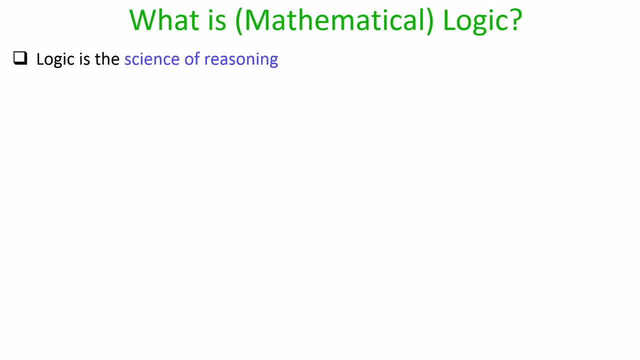 is mathematical logic. So, on a very high level, mathematical logic is the science of reasoning, So it tells you how to verify or how to conclude whether a statement or mathematical statement is true or mathematical statement is false. To be more precise, ah, consider this: 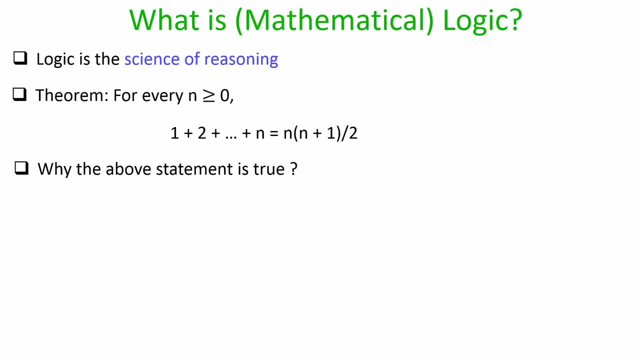 theorem statement ah, which is a very straight forward theorem statement ah, which says that for every n greater than equal to 0, the summation of first n numbers is n times n plus 1 over 2.. So this is a mathematical statement. and now 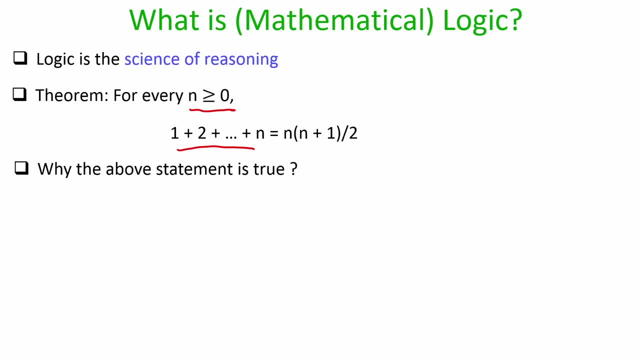 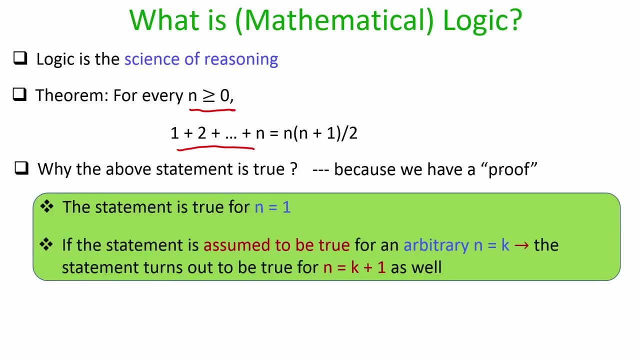 we want to verify whether this statement is true or false. Well, it turns out that this statement is true because we have something called what we call as proof, and there are several proofs for proving this statement to be true. So one of the simplest proofs: 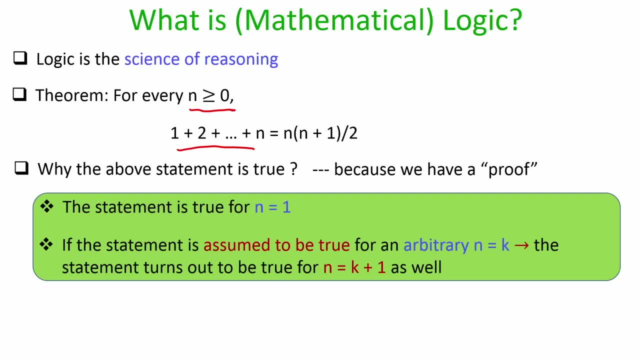 ah, is the proof by mathematical induction. So the proof by mathematical induction basically argues that the statement is obviously true for n equal to 1. and then we show that if we assume, if we assume that the statement is true for any arbitrary n equal to k, then 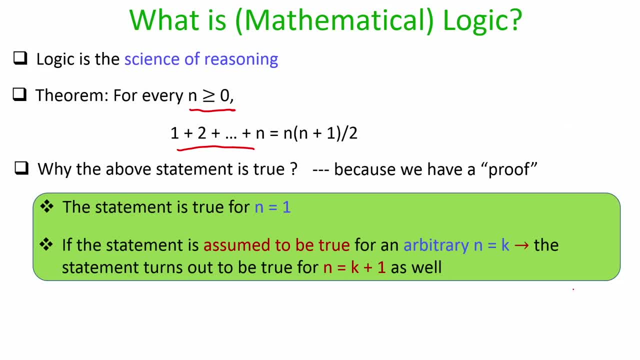 we also end of showing that the statement is true for n equal to k plus 1 as well, And these two statements constitute of proof and based on the above two points, we conclude that our theorem statement that we made here is true. Now the question here is on what? 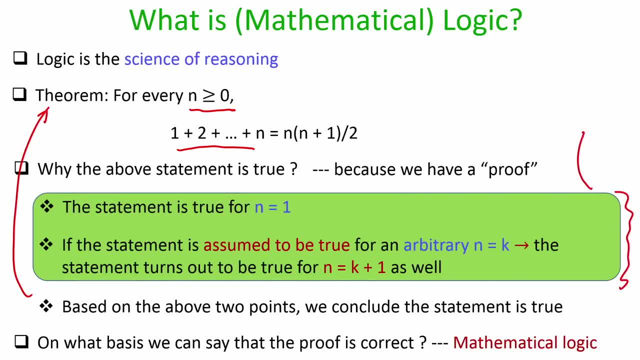 basis, we can say that these two statements that we have written here in this highlighted rectangular box constitutes a correct proof. right, how do we argue that? indeed, this is a correct proof. So, on a very high level, mathematical logic or the science of reasoning is what helps. 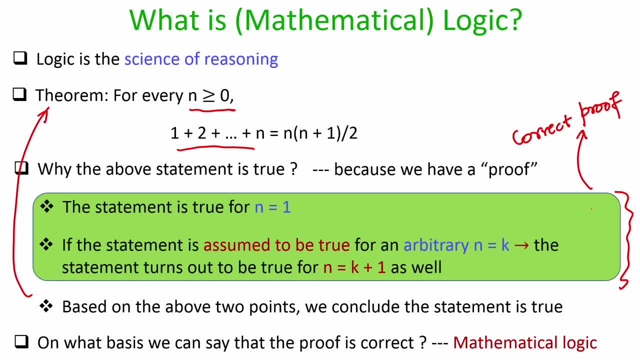 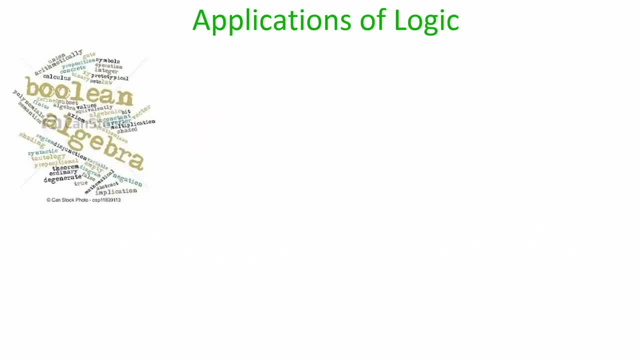 us to conclude that the two statements that we have written here indeed constitutes a valid proof for proving that the statement is correct. It turns out that there are several applications of logic, So, for example, we use it extensively in Boolean algebra, which forms the basis of computer. 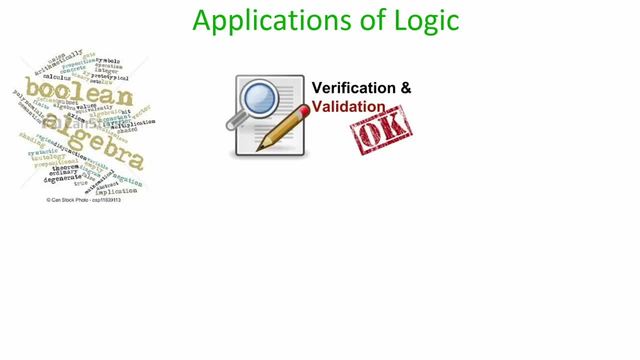 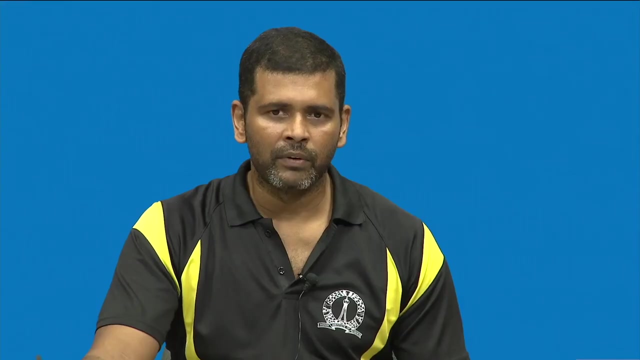 architecture. we also use it for verification, program verification and validation. So what I mean by program verification here is the following: suppose we have written a software for particular application, how do we verify whether our software is performing is intended task? One way of verifying that is we run the program or the software. 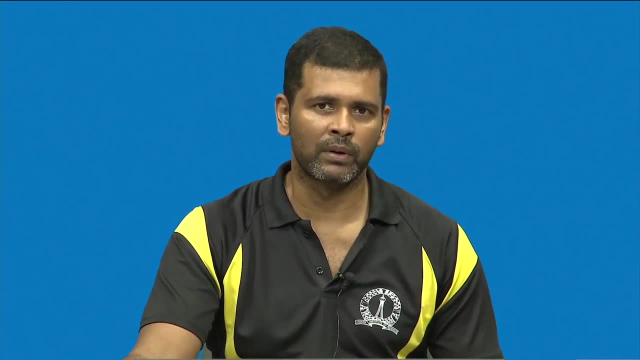 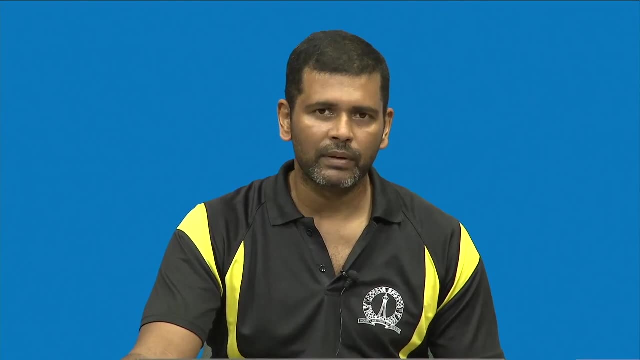 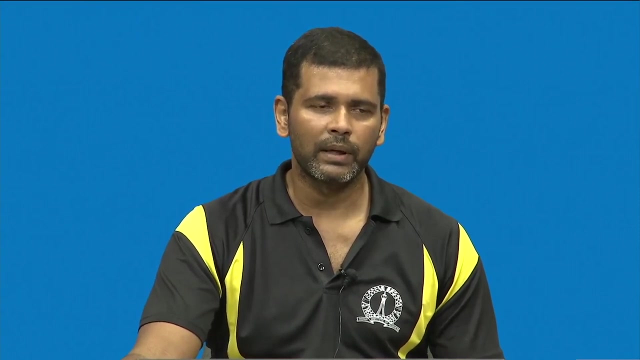 For various inputs and verify whether it is giving the correct output or not. and if it is giving the correct output for various inputs that we have tried, then we get a belief that we believe that the program is indeed performing its intended task. But in this process there might be a possibility that there is some bad input- we never which. 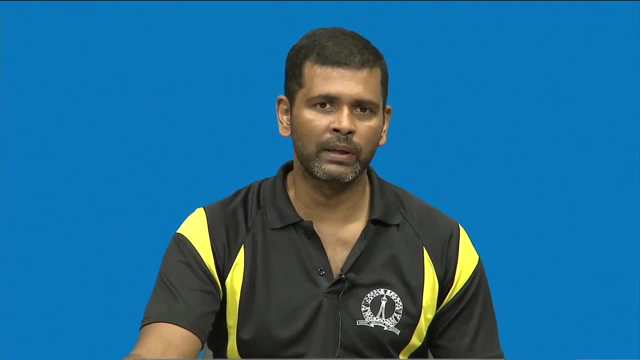 we never tried right, for which the program may not be performing or may not be giving you the right output. So this way of verifying the program is not the right way. So this way of verifying the program is not the right way. So the only way we can implement this approach- this is the one way we could do- it- is the 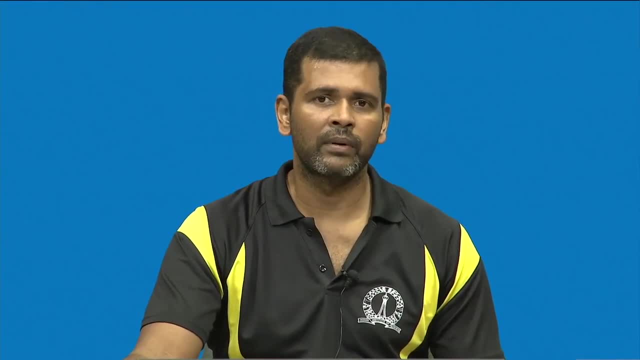 world data approach specifically for softwares or programs which are meant for very critical applications. So, for example, if your software is developed for airplane application, then we require the software to be completely robust. it should be full proof. it should, it should perform. 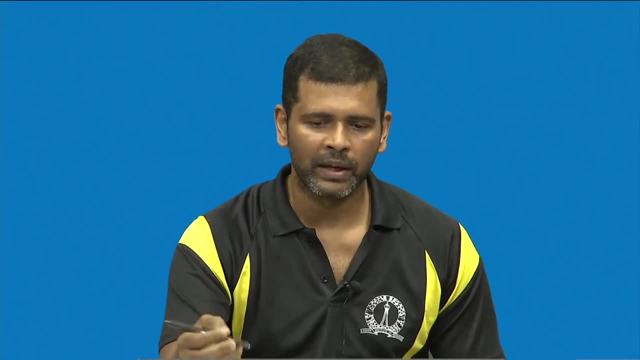 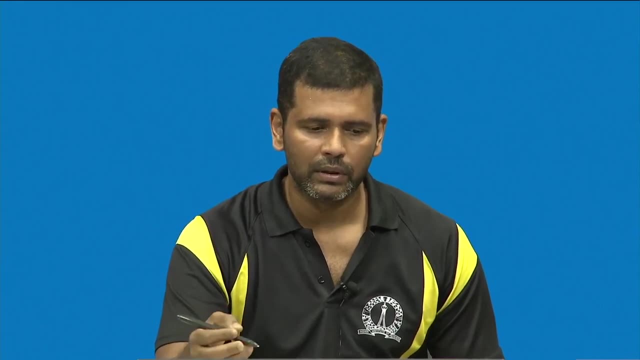 its actions always correctly. So there we use mathematical logic to verify whether the software is indeed performing its right task or not. So there is a huge body review we have done, body of work or discipline of computer science which we call as program verification, and 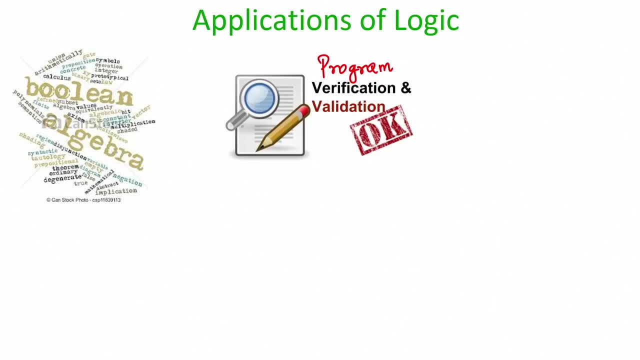 validation, where the goal is to verify whether the given software or the program is performing is correct intended application or not. So there also we use mathematical logic. The similar way we use mathematical logic for hardware verification. So for instance, if you have seen your motherboard and there are several chips or various units, 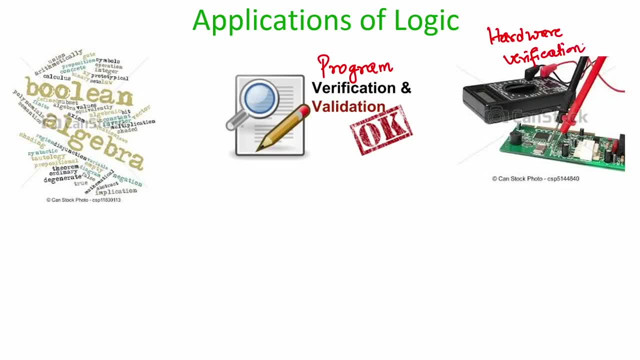 which are embedded there, which are very small in size. So how do you verify whether the embedding that you have done on your motherboard is correct or not, whether it is performing the right task or not? So, again, we use mathematical logic to do hardware verification. 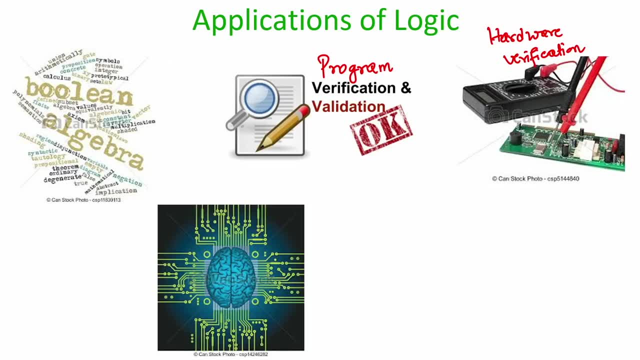 Mathematical logic is very useful in artificial intelligence. In fact, there is a programming language which is called as Prolog, which is used extensively in AI applications, and the basis for Prolog is mathematical logic. And we also use mathematical logic for proving theorem in the form of automated theorem proving. 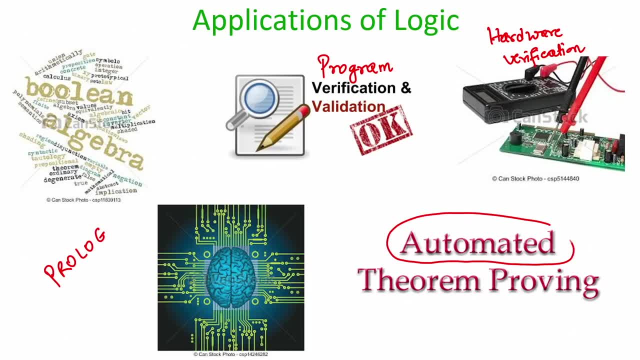 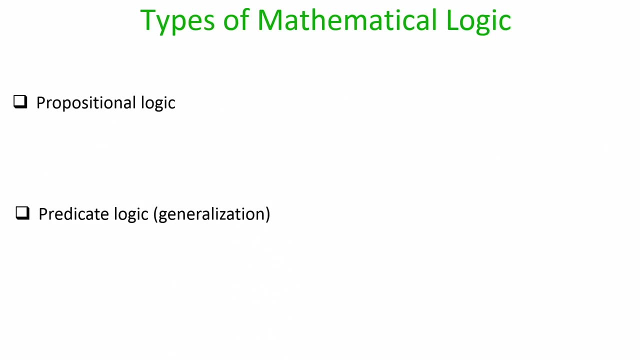 where in automated theorem proving we write computer programs to prove whether a statement is true or false. So there also we use mathematical logic extensively. So it turns out that mathematical logic is very important, very significant, And there are various types of mathematical logic. 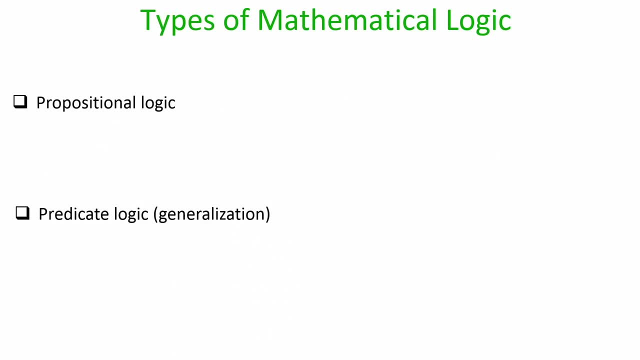 The basic form of mathematical logic is called as propositional logic, and a generalization of propositional logic is called as predicate logic. So let us begin our discussion on propositional logic. So we first define what we call. what is a proposition? So, informally, proposition is a declarative statement which is either true or false. 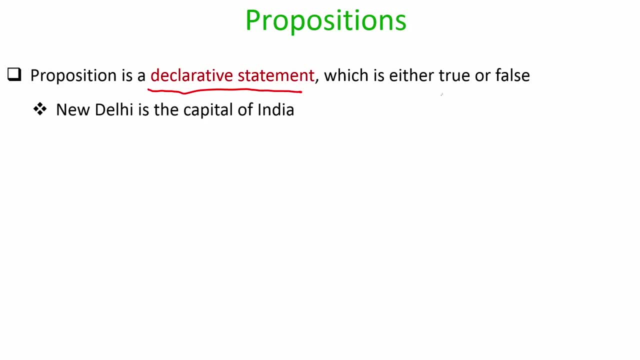 But it cannot take both the values simultaneously. That means it has to be either true or it has to be either false. So, for instance, consider the statement that New Delhi is the capital of India. It is a declarative statement because it is declaring something about the city called. 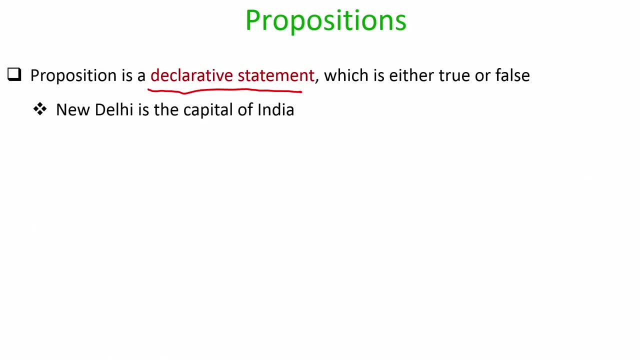 New Delhi. It is declaring that the city New Delhi is capital of India or not, And indeed the statement can be either true or false, because if you take the city New Delhi, then either it will be the capital of India or it will not be the capital of India. 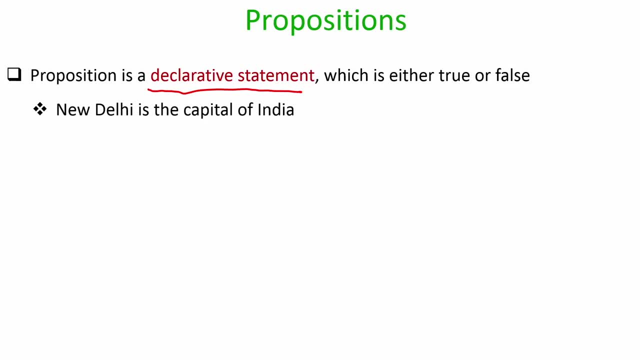 But it cannot happen. It is simultaneously capital of India as well as it is not the capital of India, So that is why it is a proposition. In the same way, if I make a statement like, say, Bahubali was killed by Kartapa, then this: 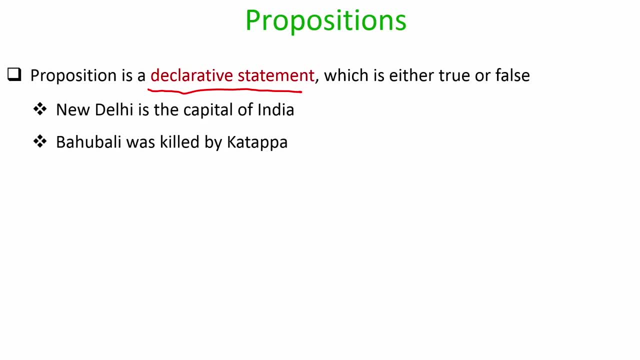 is a declarative statement because it is declaring something about a character called Bahubali and Kartapa. And this statement is indeed true because we now have a proof. whoever has seen the movie Bahubali part 2, we now have the witness that indeed, in that movie, the character Kartapa 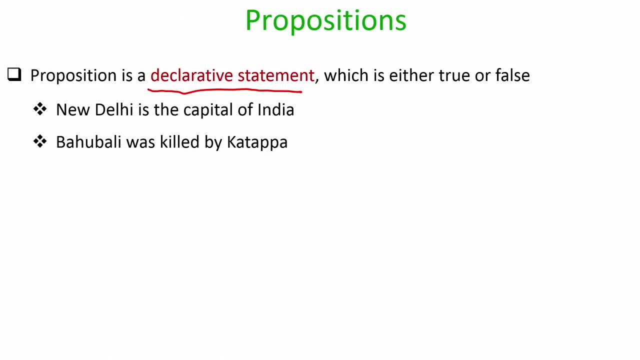 killed Bahubali, So this is also a declarative statement, Thank you. It is a declarative statement, which can be either true or false, and hence it is a proposition, whereas the statement x plus 2 is equal to 4.. This is not a proposition. well, it is a declarative statement because it is declaring something. 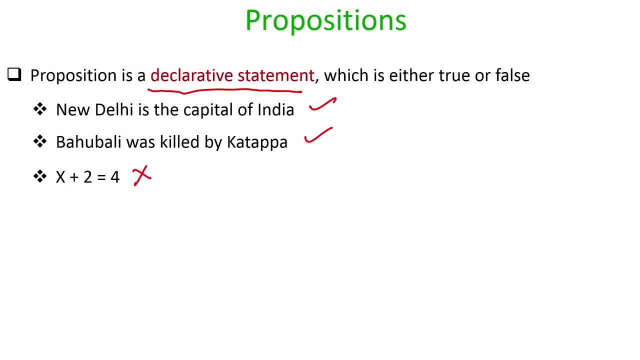 about x, 2 and 4.. But we do not know what is the value of x. depending upon the value of x, this statement can be either true or it can be either false, So it can simultaneously take values true as well as false. So hence it is not a proposition. 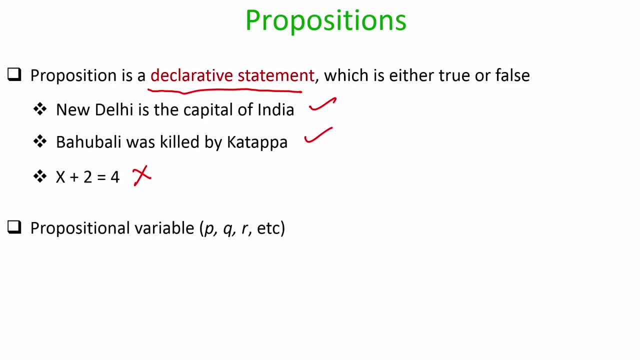 Okay, Thank you. Now let us next define what we call as propositional variables, and this propositional variables are typically denoted by lower cap letters, say, for instance, P, Q, R, etc. So what is a propositional variable? It is a variable which represents an arbitrary proposition. right, that means it is a placeholder. 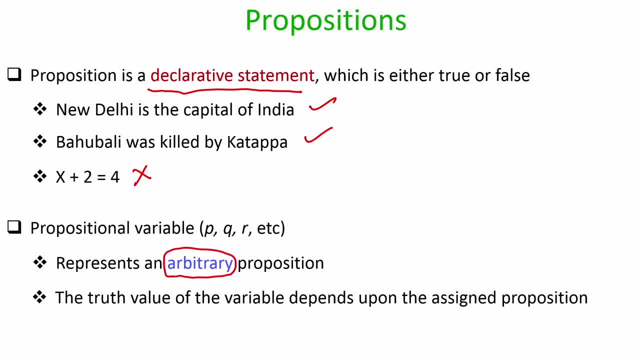 to store an arbitrary proposition and a truth. value of this propositional variable depends upon the exact propositional value. Okay, So this is the exact proposition which we assigned to this variable: P, Q or R- right? So for instance in your programming language, say, for instance in your C programming language: 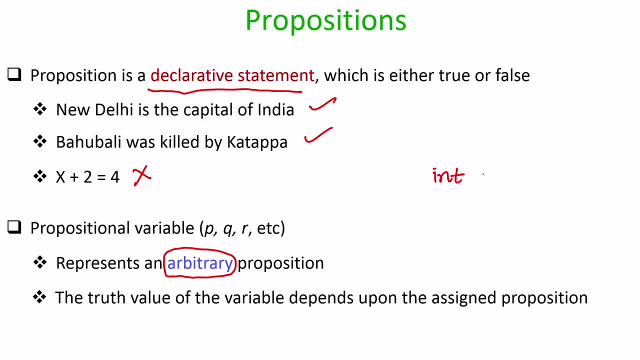 we define variables like integer variables. So if I make a statement declaration like int x, that means I am declaring here that x is an integer variable. right, and this variable can store any integer value. it can store value 1,, 2,, 3- any integer value. 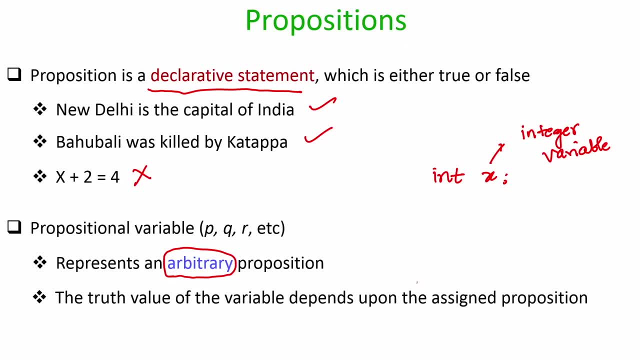 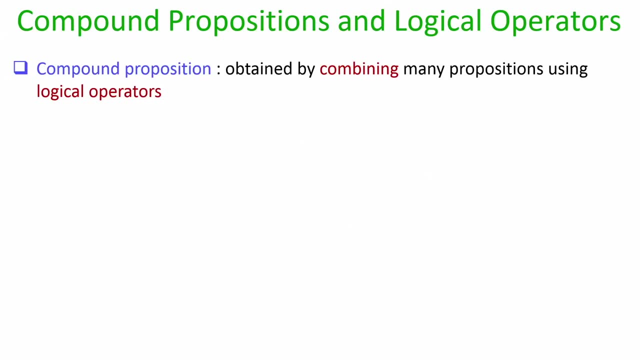 Okay, So a propositional variable. it is a placeholder for an arbitrary proposition and depending upon what exact proposition we assign to that variable, the variable can take the truth value, either true or false. Okay Now let us next define compound propositions. So a compound proposition is a larger proposition or a bigger proposition which is obtained. 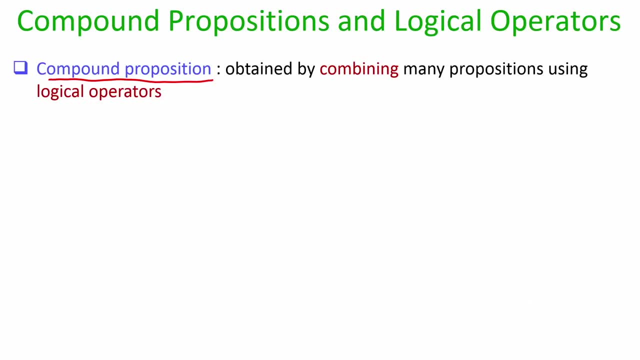 by combining many propositions, Okay, Using what we call as logical operators. Okay, So the simplest form of the logical operator is the negation operator, which is a, which is an unary operator because it operates on a single variable, and the truth table, or the 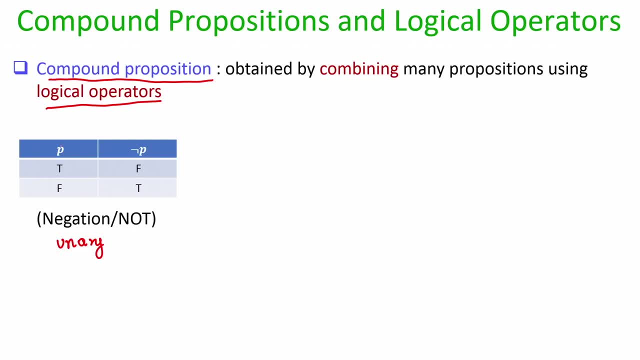 truth assignment for this negation operator is as follows: So imagine, P is a variable propositional variable and this propositional variable can take two values, either true or false. So T here stands for true, Okay, And F stands for here false, Okay. 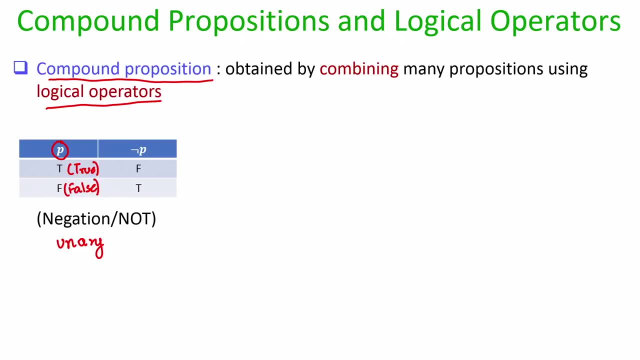 So this negation operator is defined as follows: if the variable P is true, then the negation of P will be false, whereas if the variable P is false, then the negation of that variable will be true. That is how this unary operator, negation, is defined. 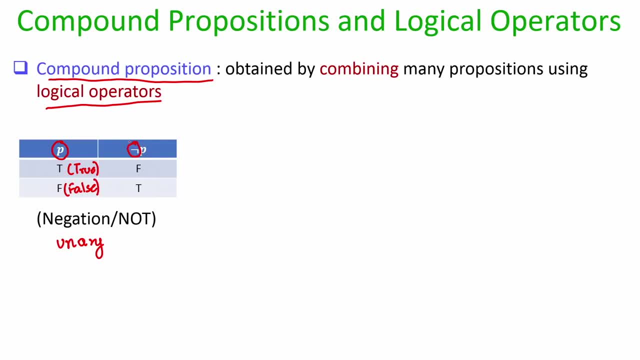 So we will be using this notation for denoting the negation operator In various other books. there are different notations which are used for the same negation operator. In some books they use this tilde symbol, tilde p, to denote negation of p. 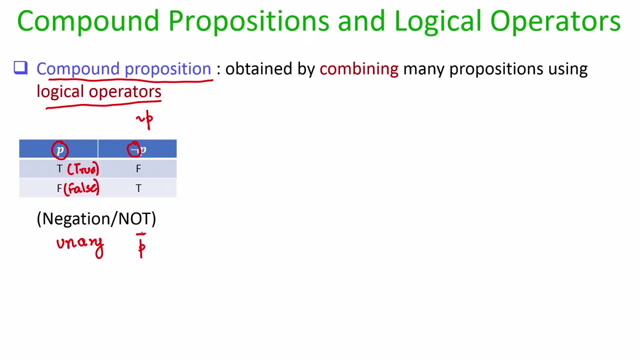 In some books they also use this p complement. that means we put this bar on top of p. So there are various notations for the same negation operator, but we will be extensively using the notation that is there in this table. Now we define another logical operator which is called as the conjunction, and it is also 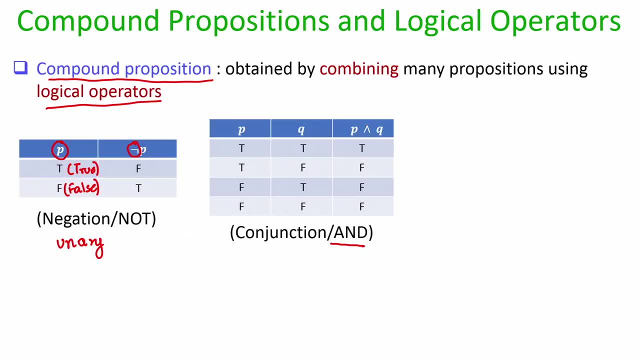 called as and logical, and, and we denote this operator by this notation. Again, in some books they use the notation p, dot q, but I will be using the notation p and this inverted this symbol q. ok, And this is a binary operator because it operates on two propositional variables. 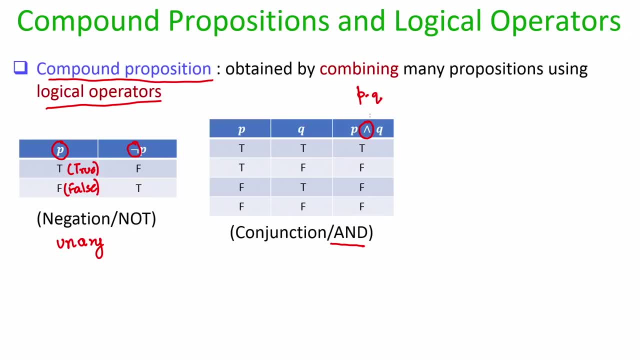 So if your p is a variable and q is a variable, then p conjunction q is another propositional variable and the truth value of p conjunction q is defined as follows: P conjunction q is defined to be true only when both the variable p as well as the variable. 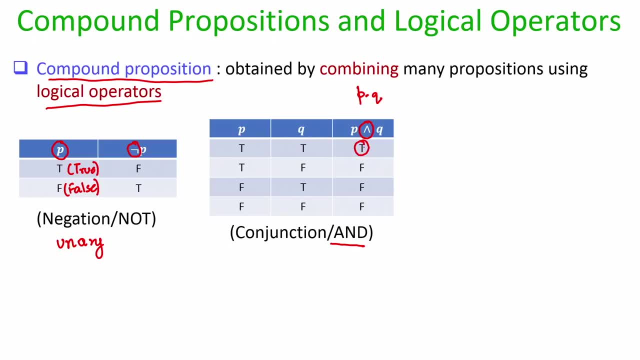 q are simultaneously true. If any of them is false, then the conjunction of p and q is defined to be false. The next logical operator is the disjunction operator, which is also called as R operator, denoted by this notation, and it is defined as follows: 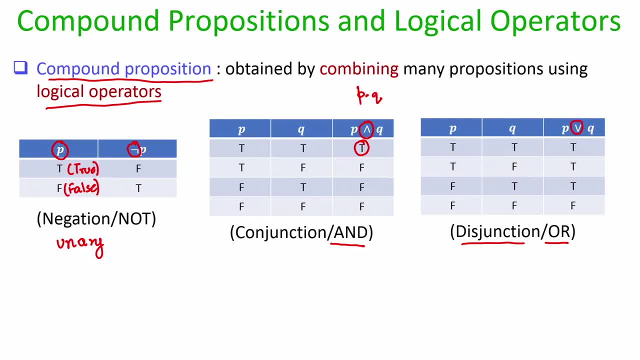 If any of the variables p or q is true, then the disjunction of p and q is defined to be true, but if both p and q is false, then the disjunction is defined to be false. ok, And it turns out that there are plenty of other logical operators that we can define. 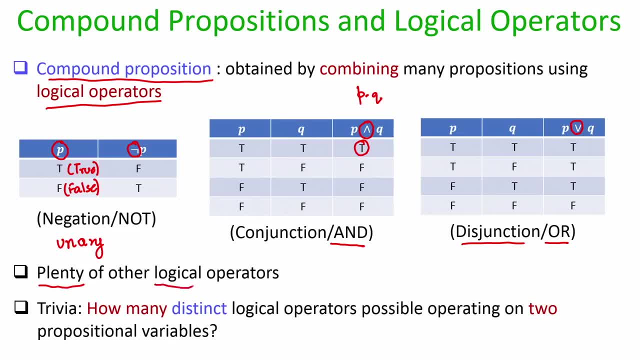 it on propositional variable, By the way. why I am calling them as logical operator? because it is operating on propositional variables. that is why I am calling it as logical operator, and the result of any logical operator will be either true or false, because we are in two valued logic, where the propositional variable or the result 0'31". maar ee0, na8, R- tu 05.oc0,- a k embed ma3 uzxk 3, 0'2 a di0, a n sí 바�c 3'. a segue: chorea R 0,2.00, long of s x Such czł RA 하게 C 0, V 0, W, Z x, q 8, R U, zk doh xsx2, tp ab n 0' historia, q, dFO & E binary Passover. 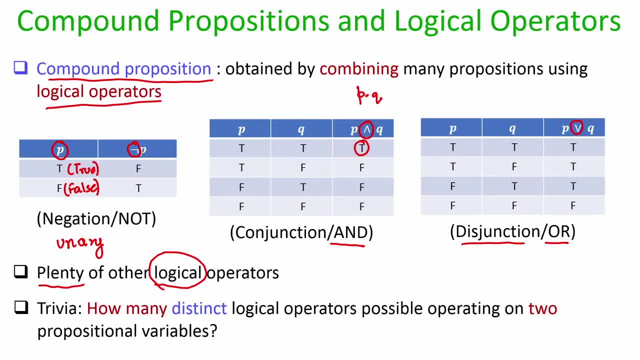 operator can take only one of the two possible values. Now here is a question: how many distinct logical operators are possible operating on two propositional variables? that means, suppose I have propositional variable P and a propositional variable Q. my question is how many distinct types of logical operators I can define on these two. 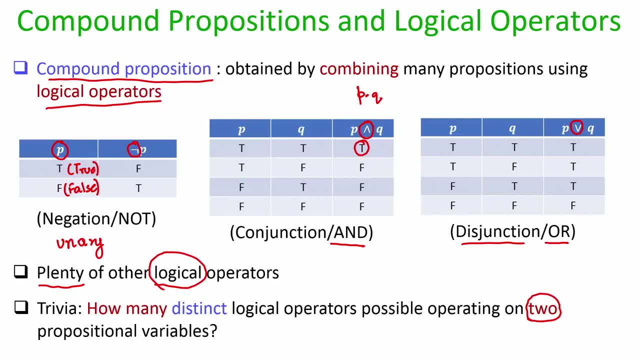 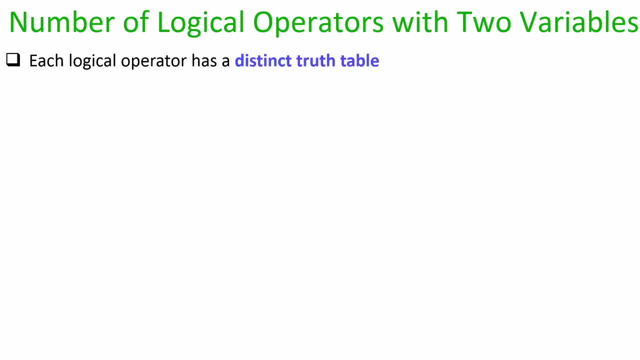 propositional variables. So you can think in your mind and try to come up with the answer. let us try to derive the answer for the question. So to begin with, you should understand that each logical operator has a distinct truth table. that means it does not matter what is the name of the logical operator that you 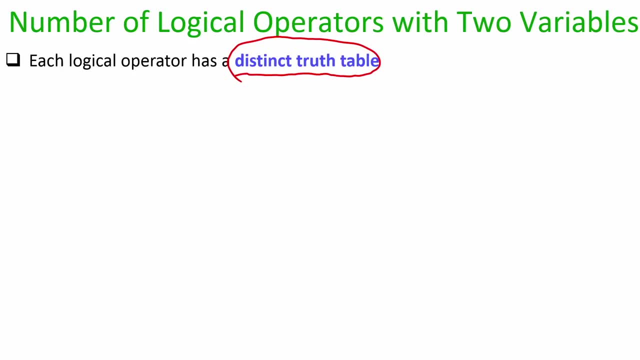 give. you can call it conjunction, disjunction x, y, z, alpha, beta, gamma, you can call it by any name. Once you fix the name of a logical operator operating on variables P and Q, then it has a distinct truth table. and what do I mean by a distinct truth table? well, since we are 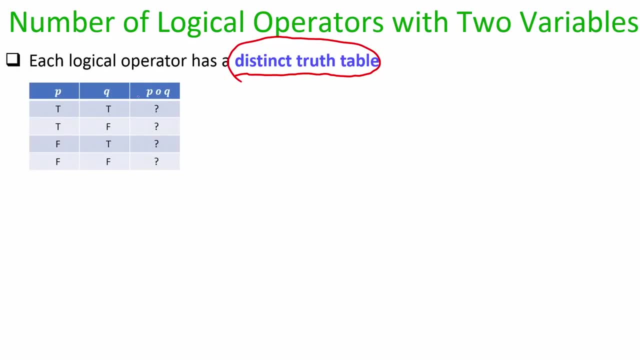 trying to define a logical operator on two variables, then the variables P and Q can take these four combinations right: P can be true, Q can be true, P to be true, Q to be false, P to be false, Q to be true and P to be false, Q to be false. 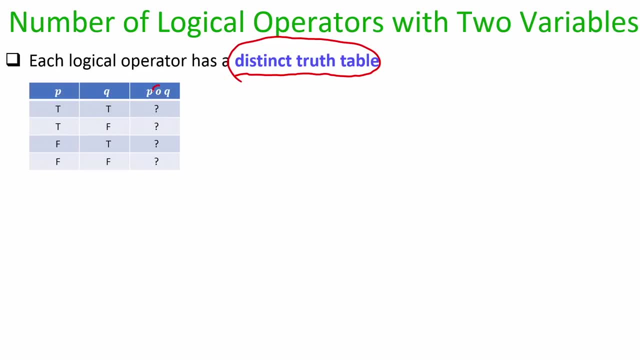 So we have these four possible combinations, and here O is denoting by arbitrary propositional variable. ok, My goal is to identify how many different types of arbitrary logical operator O I can define here. right, that is my question here. And the question marks here denote what will be the truth value of P operation Q for the. 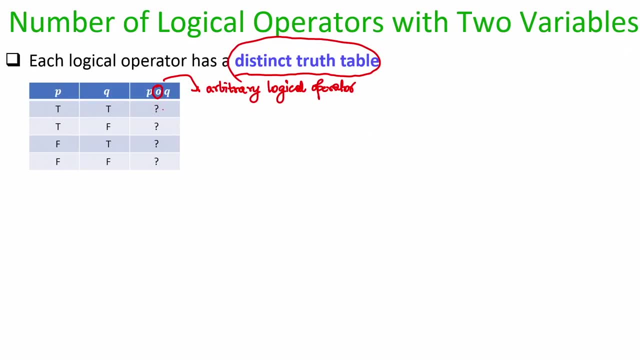 various truth assignments. That means here: the first question mark says what can be the possible value of P operation Q if both P and Q takes the truth value true. The second row here denotes what is the value of this operation operator, P operation Q, if P takes the value true, Q takes the value false, and so on. 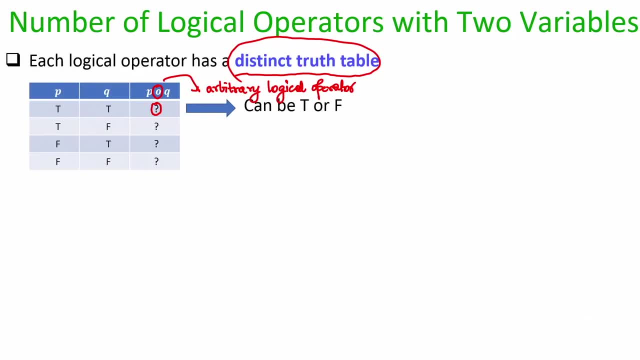 It turns out that since we are dealing with mathematical logic, where each variable can take only two possible values, then each of these possible question marks can be either true or false. That means my operation O can be such that for P to be true and Q to be true, the result 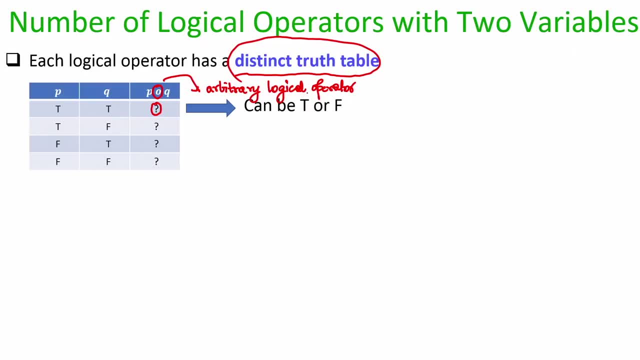 of P operation Q can be either true or it can be either false. In the same way, my operation O can be such that for P to be true and Q to be false, the operation P, operation Q may result in true or false, and this holds for all the four possible. 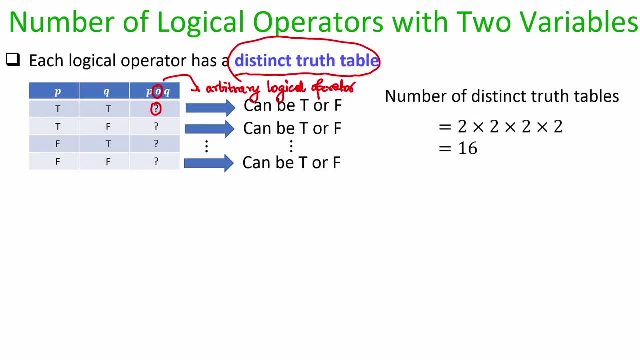 rows. It means that if I consider the number of distinct truth tables, Ok, Here I can construct at most, in fact, exactly 16 distinct truth tables, because for each of the possible rows here, for each of the possible question marks here, I have two possible options. 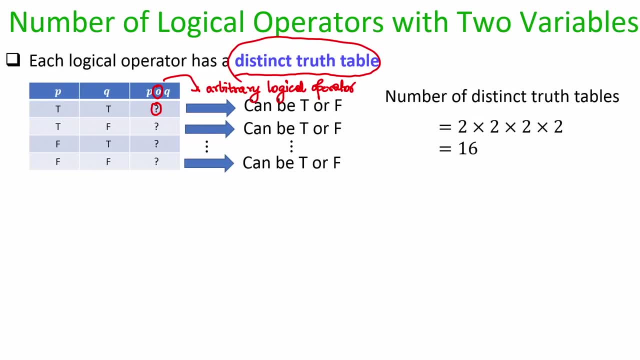 and each of them is independent of each other. each of them are independent. So that is why I have total 16 number of distinct truth tables possible. sorry for this rendering issue here. this parenthesis should come down here. So, since each row should take the value true to or false, that is how I get a total number. 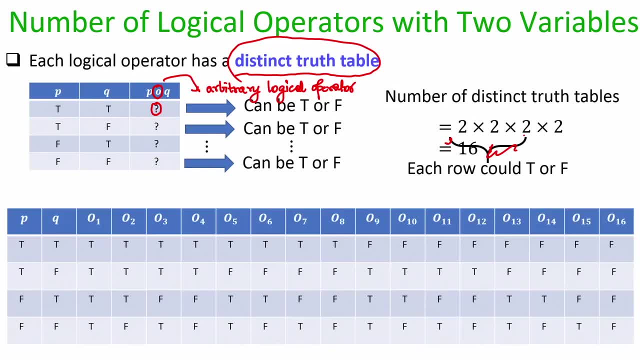 of distinct truth tables to be 16.. And what I have done here is I have written down the 16 distinct truth tables which can be possible. I am calling those distinct, 16 distinct truth tables by various operators. so operator one denotes a truth table, where for 16 distinct truth tables, 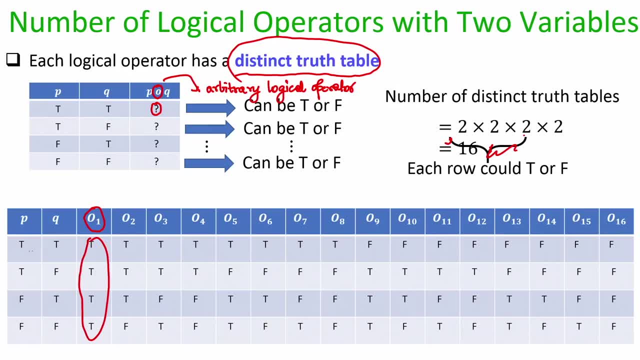 Ok, Ok, Ok. For P to be true and Q to be true, the result is true. for Q. P to be true, Q to be false, the result is true. for P to be false, Q to be true, the result is true. and for P to be false, Q. 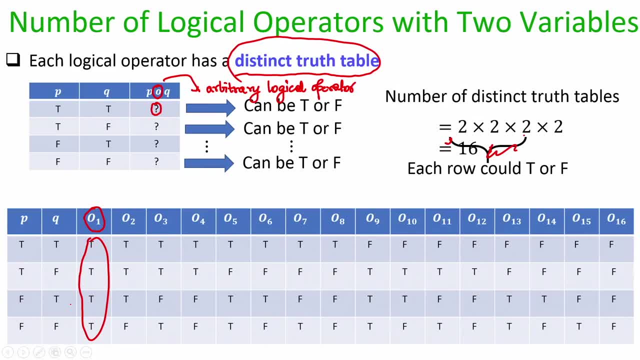 to be false. the result is true. That is one possible truth table, and I am saying that that corresponding operator is operation operator O1.. Same way, I have operator O2, O3, O4 and operator O6, and now I can give fancy names to each. 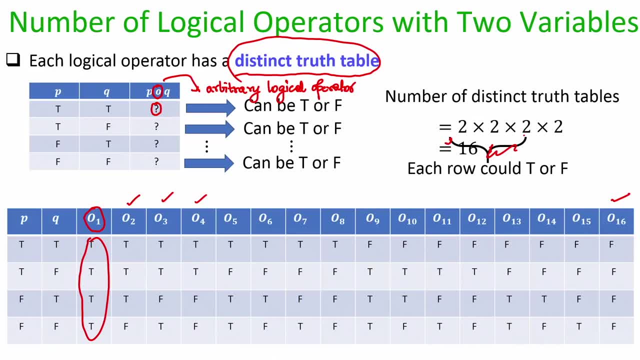 of these operators. I can give some name: Conjunction, disjunction, XOR, exclusive OR exclusive, NOR, etc. etc. But I cannot give more than 16 distinct names, because I do not have more than 16 possible truth tables Right. 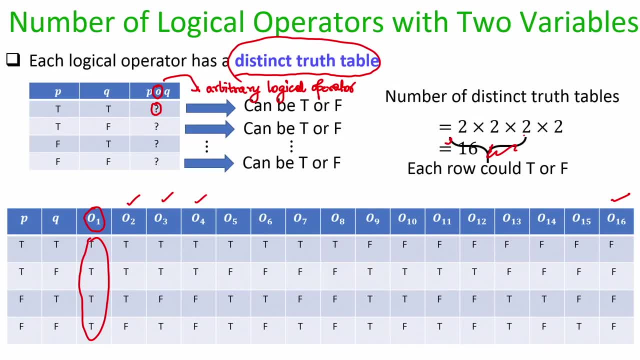 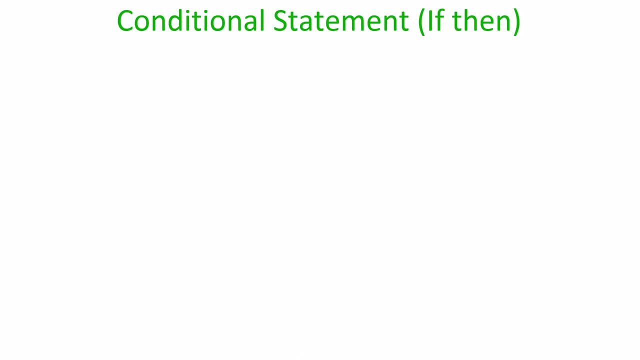 So that is why there are 16 possible logical operators, distinct logical operators which are possible with two propositional variables. Now let us define another logical operator. So let us define another logical operator, which is the conditional statement. this is also called as if then statement, and we use this notation. P implies Q and the truth table. 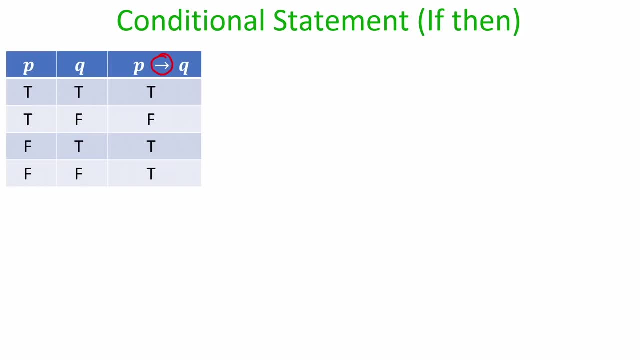 for P implies Q is defined as like follow as this: So you can see that P implies Q is true for three possible combinations and it is defined to be false only when P is true but Q is false Right Now. the question is why the truth table of P implies Q is defined like this. 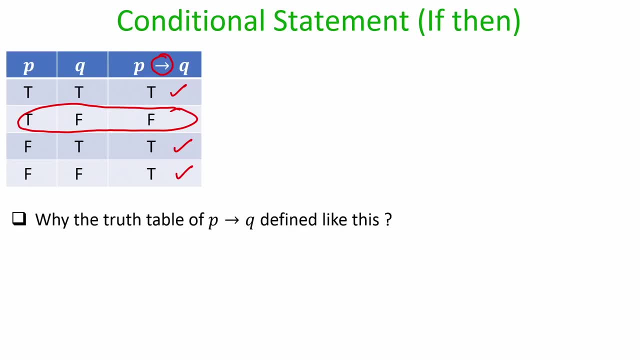 That is why the truth table of P implies Q is defined like this. That means why P implies Q is true even if both P and Q are false, or why P implies Q is defined to be true even if P is false, but Q is true. 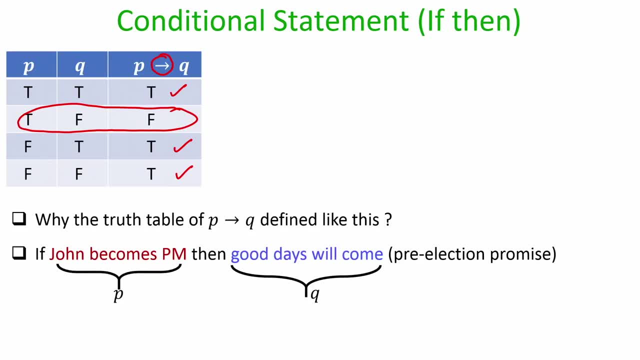 So to understand that, let me give an example, a very simple example. suppose we make this logical statement: suppose there is a PM candidate called John and he makes the election promise that if he becomes the prime minister then good days will come for the country. 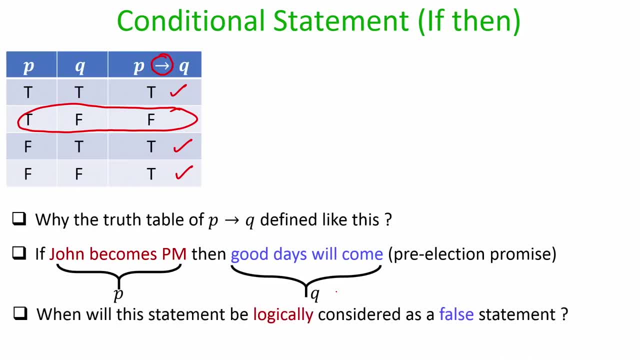 This is a pre-election promise which John makes. Now the question is: when exactly will you consider this logical statement to be false? It turns out that this logical statement will be considered as a false statement only when good days does not come, even if John becomes the PM. 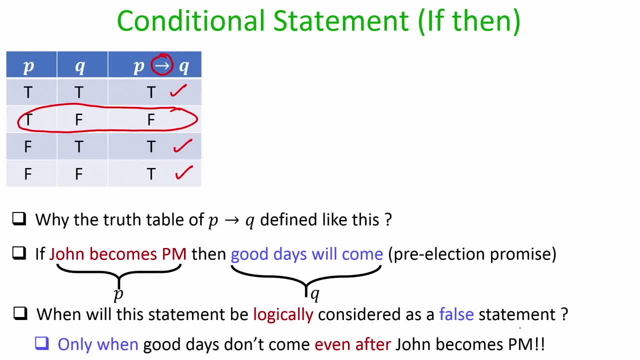 For all other cases, the statement will be considered as a true statement. That means if John does not become the PM at the first place, then I do not care whether good days come or not. overall, the statement will be considered as a true statement because John is not breaking his promise. 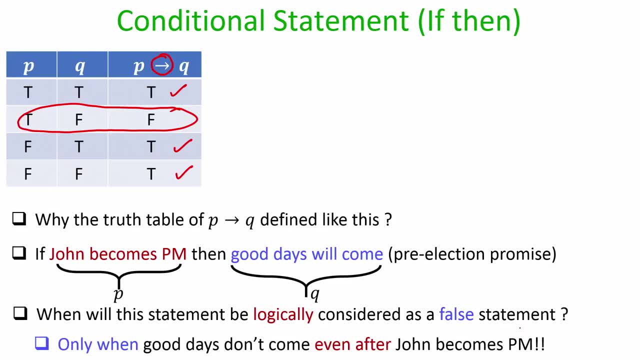 We will be considering. we will be saying that John is breaking his promise only when John becomes PM. but still, good days are not coming for the country. and that corresponds to the truth, assignment P to be true and Q to be false and, as a result, for that combination. 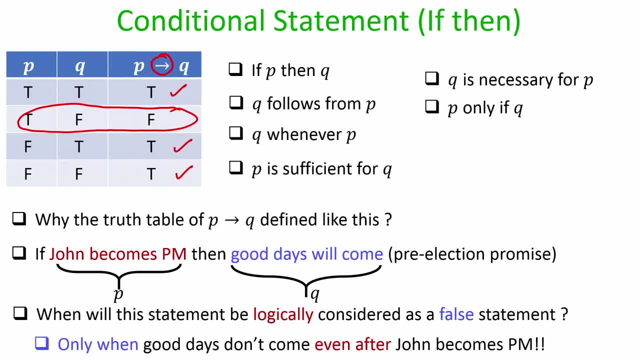 I define P implies Q to be false. There are others. There are other interpretations of this: if, then statement. So the usual interpretation of P implies Q is this: if P, then Q. but there are other interpretations like Q follows from P. So Q follows from P means if you ensure P to be true, we can. 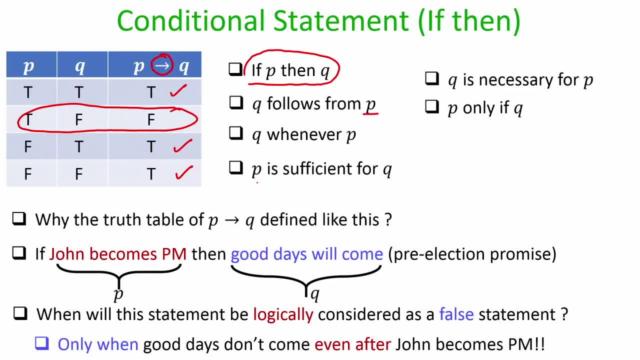 denote, we can come to the conclusion Q. P is sufficient for Q. It tells that if you ensure that P is happening or P is true, then the conclusion is Q, Q whenever. P is another way of interpreting. if P can, then Q. The question is why P implies. 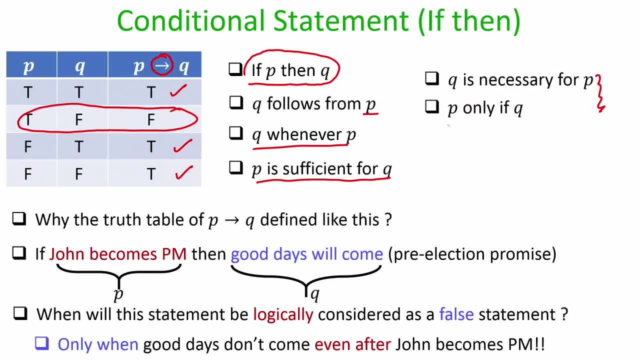 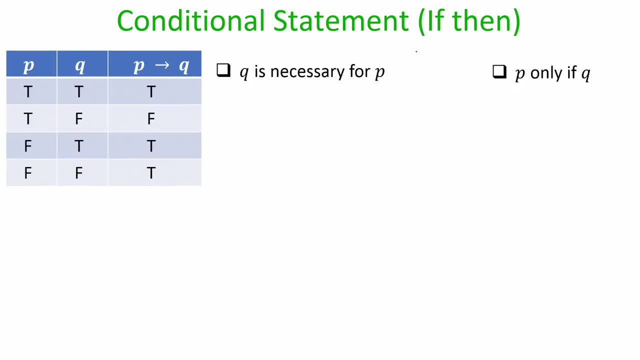 Q denotes Q is necessary for P, and why P implies Q denotes P only if Q. So these are the two common form of P implies Q, which is a common source of confusion for the students. So let us try to understand that. that why P implies Q, or why if P, then Q can also be. 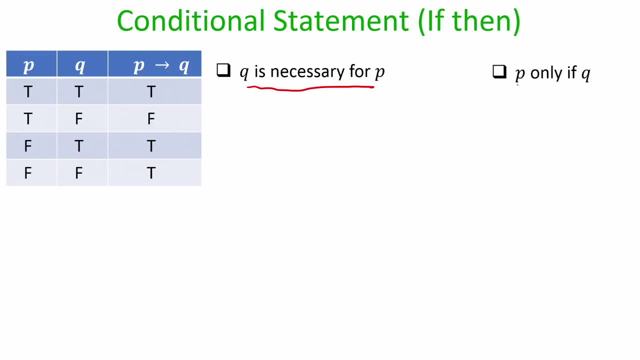 interpreted Q is necessary for P and why it can be interpreted as P only if Q. So to understand that, let me first claim here that the statement P implies Q and the statement negation Q implies negation P are both logically equivalent. What I mean by both are logically equivalent is that you 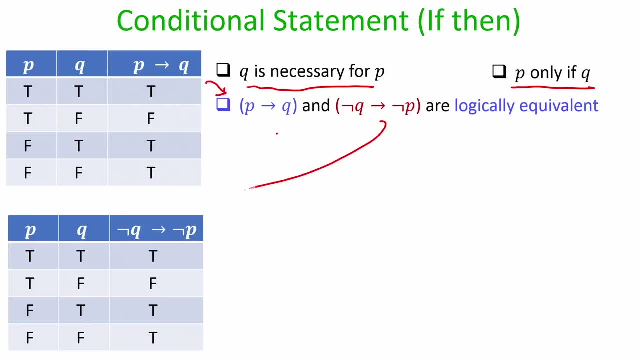 have the truth table of P implies Q and this is the truth table of negation. Q implies negation P and you can see that both of them have the same truth table. that means both P implies Q as well as negation Q implies negation P have the same truth table. So if P is Q, 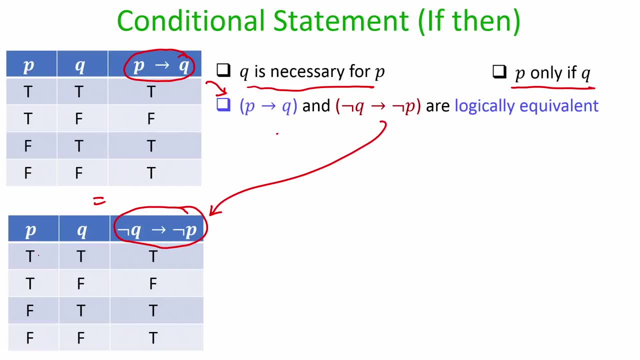 Q is true, then P implies Q is true and same is same is the case for negation Q implies negation P. that means row wise: the first row here and the first row here are same row wise. the second row here and here are same, Same row wise. the third row of the two tables are same and row wise the fourth rows of both. 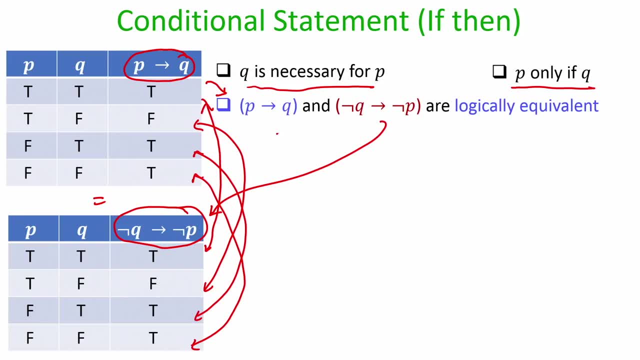 the tables are same and that is why I can say that P implies Q and negation Q implies negation P are both logically equivalent. Now consider this statement: I make the statement. my statement is: I will go to pub only if it is a Friday and say the statement I will go. 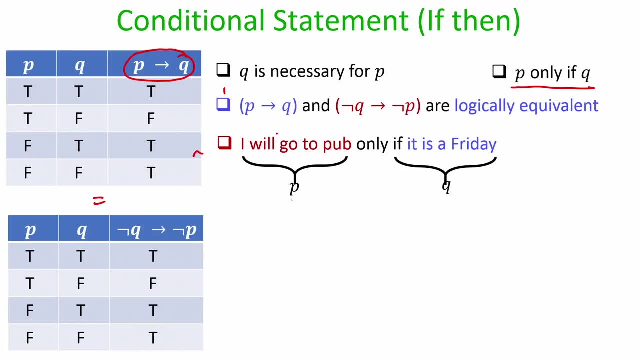 to pub is represented By P variable P. So P is a propositional variable denoting the statement I will go to the pub and Q is another propositional variable denoting the statement it is a Friday. my claim is that this statement can be represented by. P implies Q. 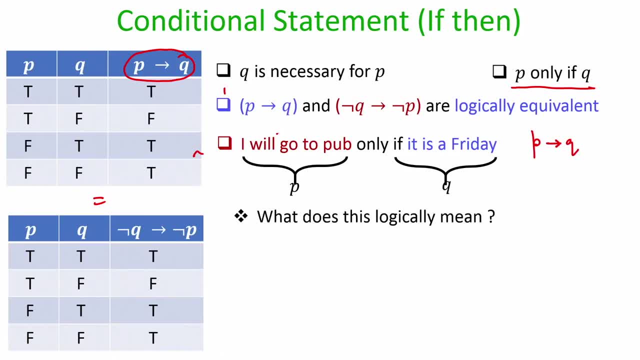 Why so? because if you try to understand the logical meaning of this English statement, then what I am trying to say here is that if it is not a Friday, definitely I will not go to the pub, because that is how the interpret, that is how the statement only if is interpreted. 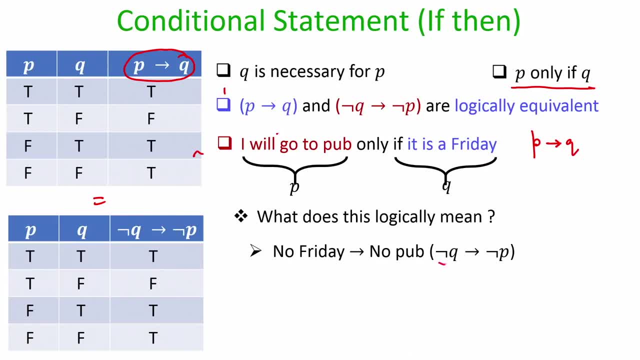 and no Friday implies no pub can be represented by negation Q. implies negation P because I am representing it is a Friday by the variable Q, So it is not a Friday will be represented by negation Q and I will not go to the pub. will be represented by negation of P because 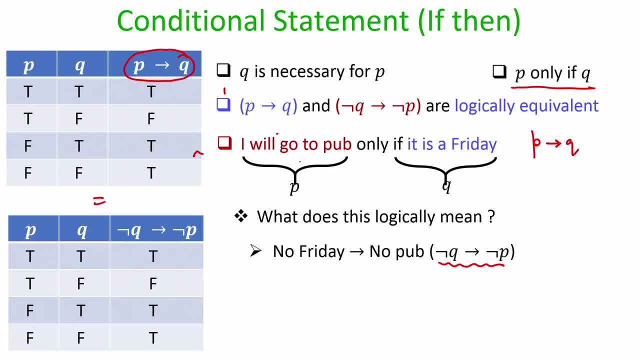 P, as for my definition, denotes hours. I will go to the pub, right. So in that sense, right Friday is necessity, or it is a necessary condition for thinking of going to the pub. that means I will think about going to the pub only if it is Friday. if it is not a Friday, definitely I would not go to the 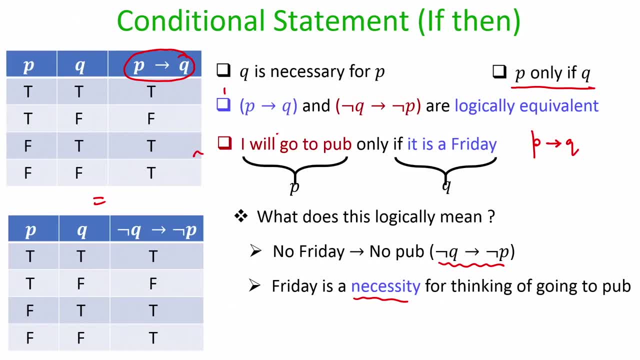 pub. So that is why Friday is a necessary condition here. but Friday is not a sufficient condition for me going to the pub, because it might be possible that there is some Friday on which I am ill, or the I have may have some personal work for which I am not going to. 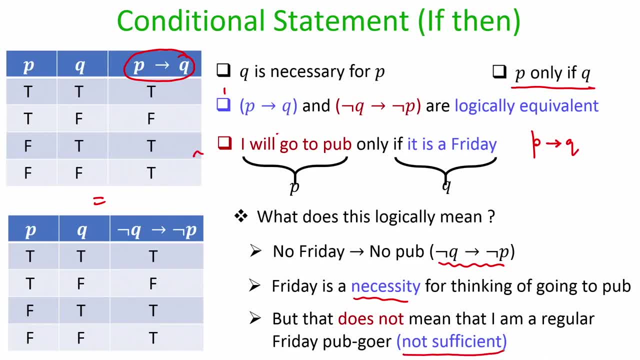 the pub. that means, in this case, being Friday- is not a sufficient condition. that means you cannot simply conclude that so since it is a Friday, definitely this guy will go to the pub, and that is why the statement I will go to the pub only if it is a Friday will be. 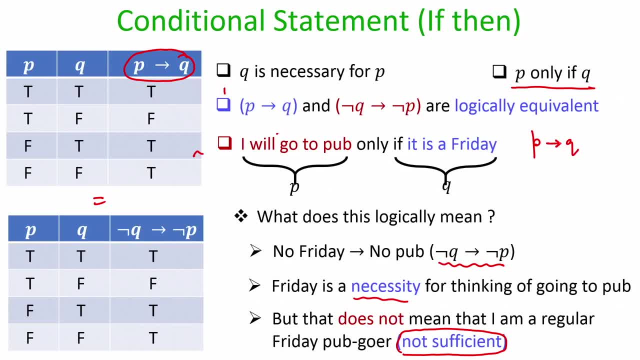 represented by P implies Q. It will not be a condition for me going to the pub, because it might be possible that it will not be represented by. Q implies P, because Q implies P denotes that if it is Friday then I will go to the pub. but that is not what I want to represent here. I want to state: 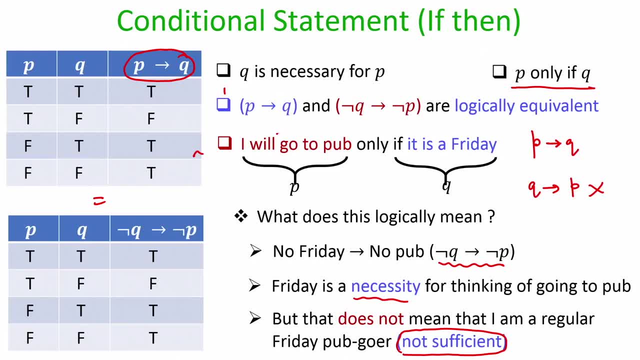 here the necessity of the condition that it is a Friday. then only I can think of going to the pub, and that is why the statements of the form that Q is necessary for P or the statements of the form P only if Q are represented by P implies Q. 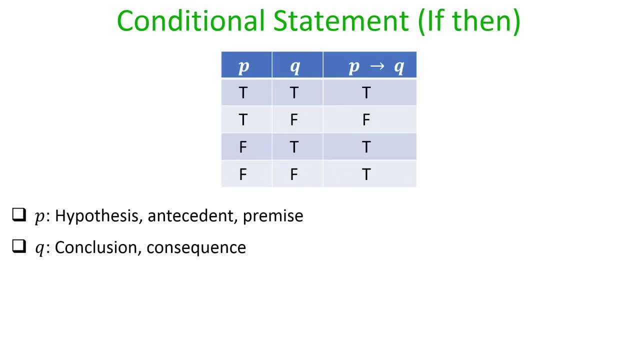 So whenever we write a conditional statement of the form, if then P implies Q, then the P statement or whatever statements you have for the propositional variable P, they are called as hypothesis or antecedent or premise, and Q denotes the conclusion or the consequence. 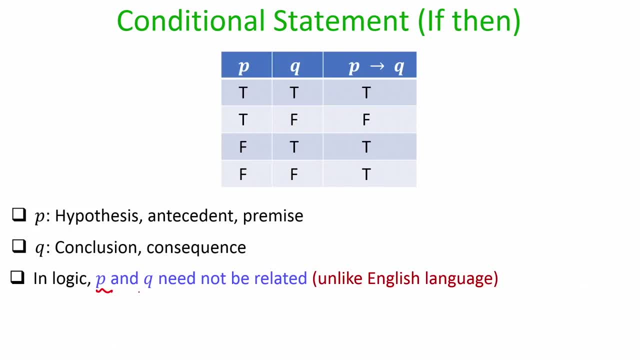 It turns out that in mathematical logic the statements in P and Q need not be related in the English sense. So, for example, if I make a logical statement that if earth is triangular in shape, then Dr Ashish, namely myself, is the director of triple IT Bangalore.